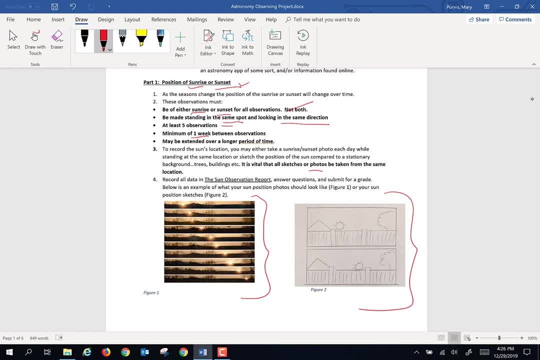 photos. Please make sure that you are standing in exactly the same spot, looking in exactly the same position, and I highly recommend that you do something to assist yourself, like lean against a fence post or put your phone on top of a mailbox, or something to make sure that you are getting. 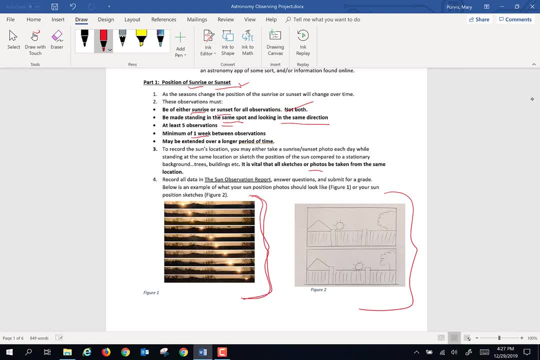 the same perspective. This is a collection of photos that I found, and you'll notice that the trees are all lined up. This tree is all lined up. This hill is all one on top of another. What you're going to do is you're going to stand at the same spot and you're going to look at the 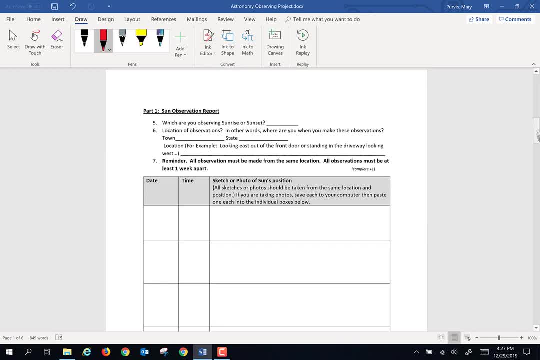 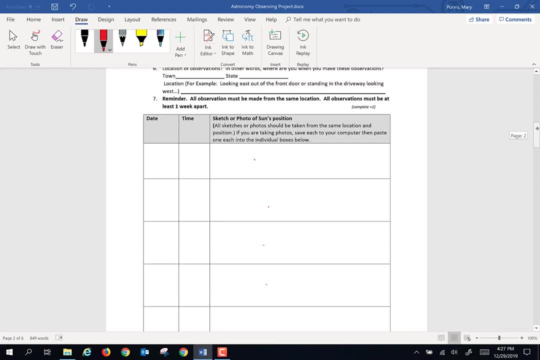 tree from the background in the same spot. The first thing you're going to do is you're going to turn into the photos Now, your photos one after another. you can upload them here or you can attach them on a separate piece of paper. You are also going to include the date and the time of. 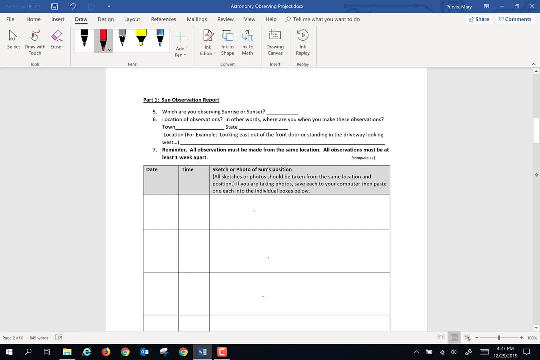 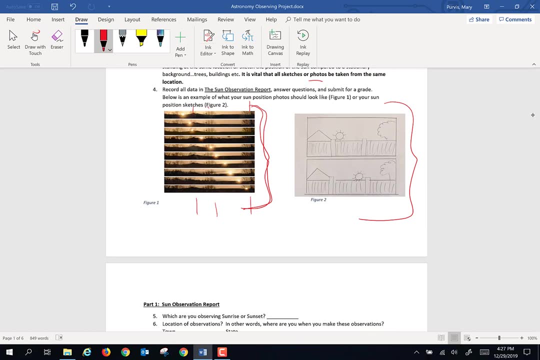 every observation, and what I want you to notice is: what direction did the sun- rise or sunset- move over time? Is the sun moving towards the north, or is the sun moving towards the south? or did it reverse directions? And it does do that Now, if cell phones and photos are not your thing. 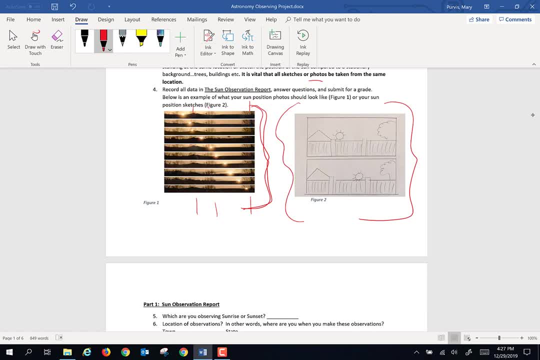 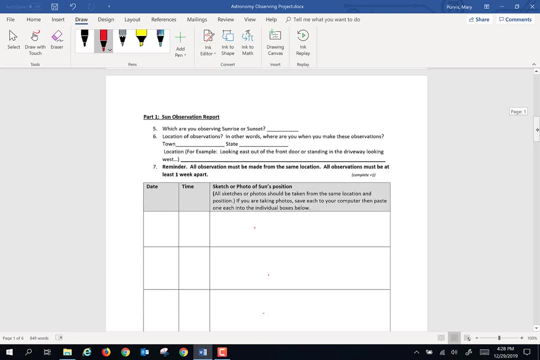 you are welcome to do this by simply making simple sketches. Please use stationary objects as points of reference: buildings, fences, trees, things that won't move. And again, you are standing in the same spot to make all of your observations When you record your. 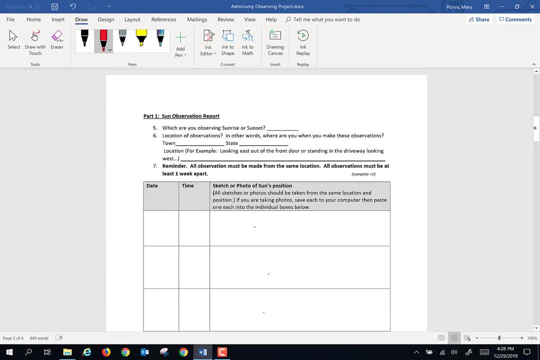 observations. which one? are you observing sunrise or sunset? Where are you making these observations? Your town, your state and your location? For example, you're looking east out of your front door, or you're standing at the end of your driveway, or you are looking out your 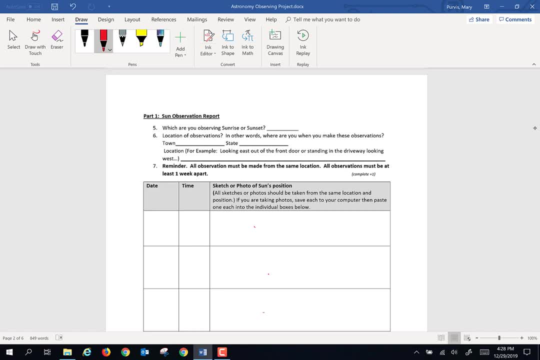 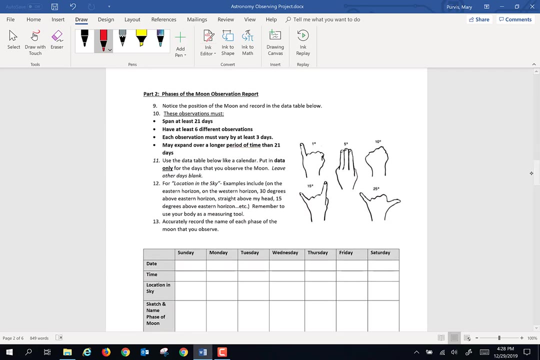 bedroom window. I don't need tremendous detail, but I do want you to know exactly what is the point of reference that you're using to make your observations. Now, when you're done with this, answer the question: what direction Did you see this move? The second part of the observing project is to ask you to look at the 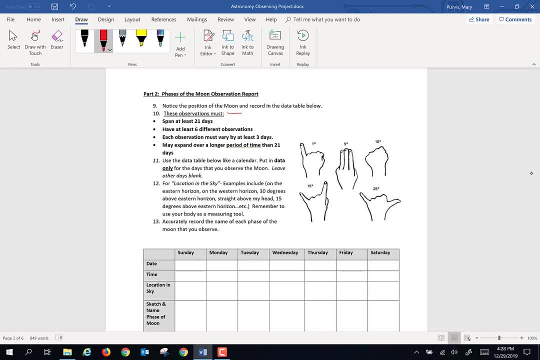 moon. I want you to observe the phases of the moon. This must be spread out at least over 21 days. I want you to make at least six different observations, and you may do a lot more. Observing the moon can sometimes be very easy to do. Each observation must be at least three days. 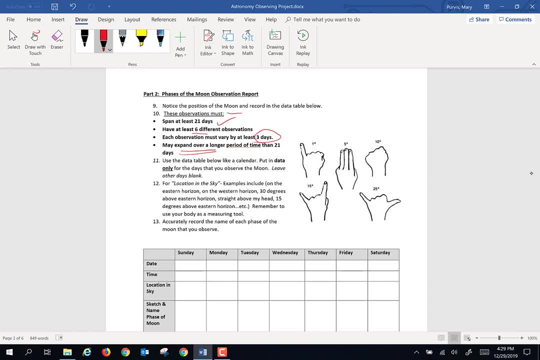 apart in order for it to be a good observation. If you have a good observation, you can make at least two wortons for each date or time. You might even measure it by measuring your date. It may be far to count as a grade. How are you going to record that data You're going to record? 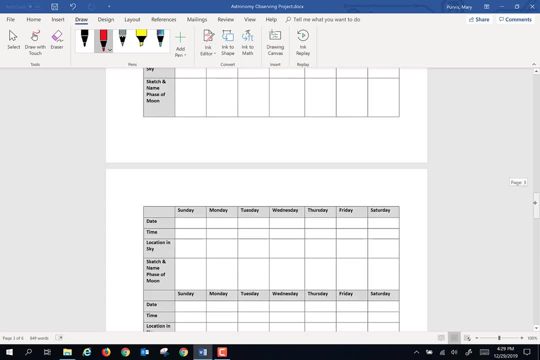 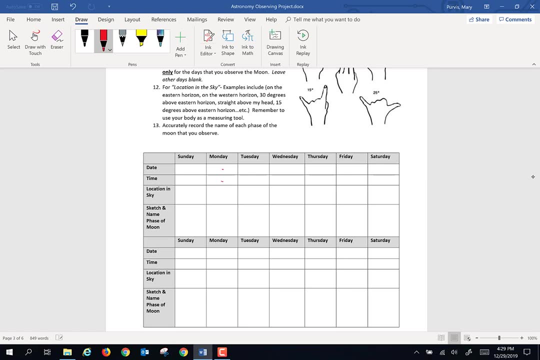 it on a data table. I made a data table for you that looks very much like a calendar. When you record the moon, you're going to put in the date, the time, the location in the sky, sketch in the phase of the moon, then sketch and then name it: Waxing, gibbous, waning crescent. 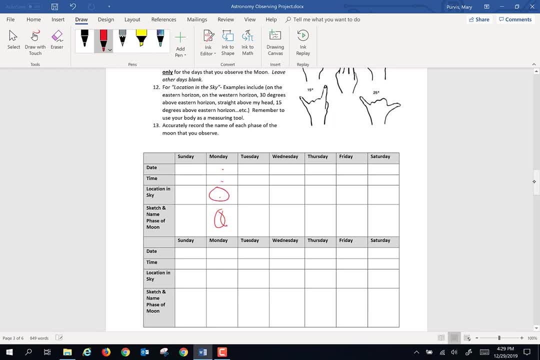 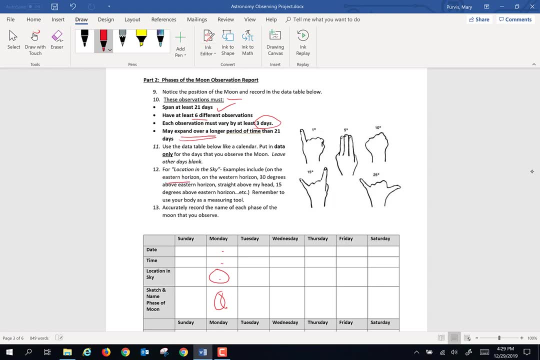 whatever it is For location in the sky, what I'm going to ask you to do is: where is it, where is the moon located? is it on the eastern horizon? on the western horizon, 30 degrees above the eastern horizon, straight above my head, at my 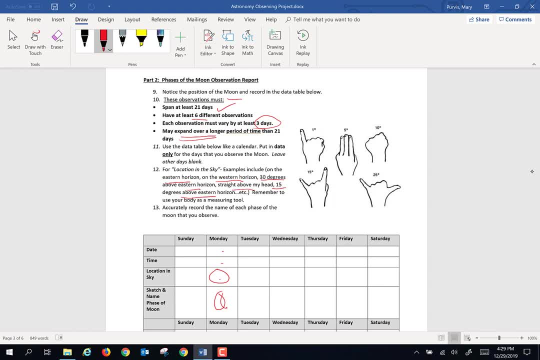 zenith 15 degrees above the eastern horizon. how are you going to measure these angles? I want you to practice. in our very first lab, you used your hands and fingers and arms to measure angles. I want you to use that skill- practice that skill- to measure these positions of the moon. 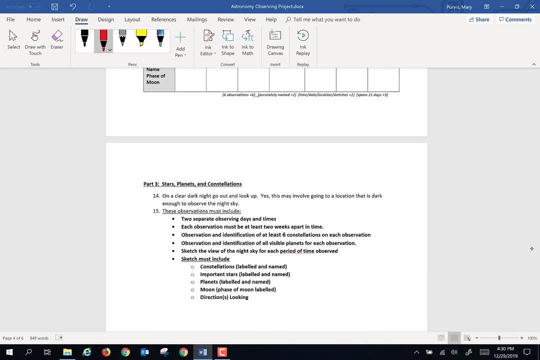 for the last part of the observing project. I want you to look at the sky and look at stars, planets and constellations. now you're going to go out and look at the stars at least two times. each observation must be at least two weeks apart and in each observation 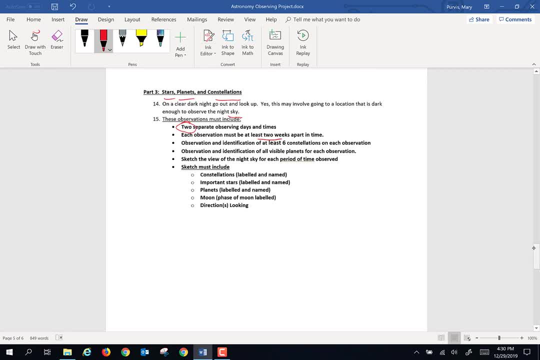 here's what it looks like, what I'm going to: ask you to record At least six constellations, any planets that are visible, and I want you to sketch the night sky for the period of time or the moment that you are actually observing the sky. You're going to sketch the constellations and label them. Write the names. 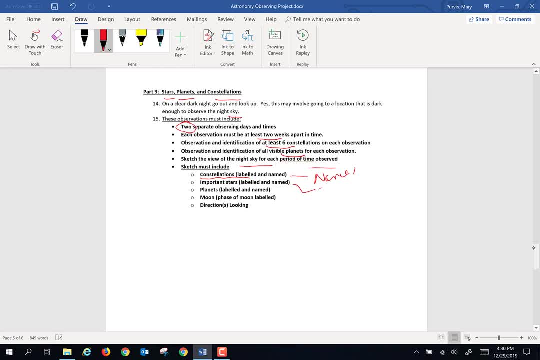 down of what constellations you are seeing. Write down the names of the important stars, like Polaris, Aldebaran, Betelgeuse. What are those important names? Are there any planets that you can see? I don't expect you to instantly know this. That's why you look things up on the 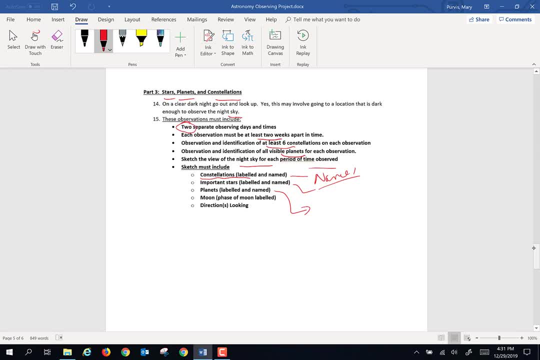 internet. That's why you use the planisphere to help locate those constellations. That's why you use an astronomy app, Find a planet and figure out what it is and label that on your observations, If the moon is out there in your observing sphere.